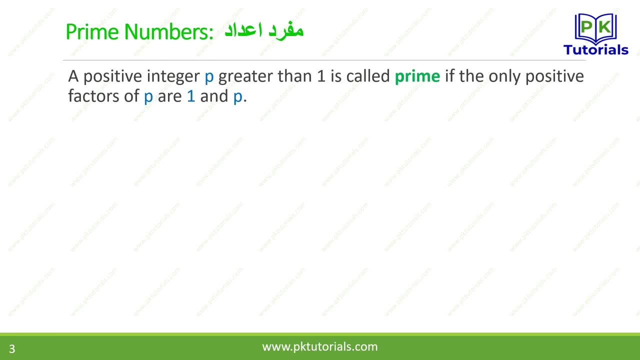 It means that any integer, if we take it and its number- sorry, its factor- is 1 or P, we call it Prime. For example, we have 3.. Let's write 3.. So what is 3?? Is it Prime or not? 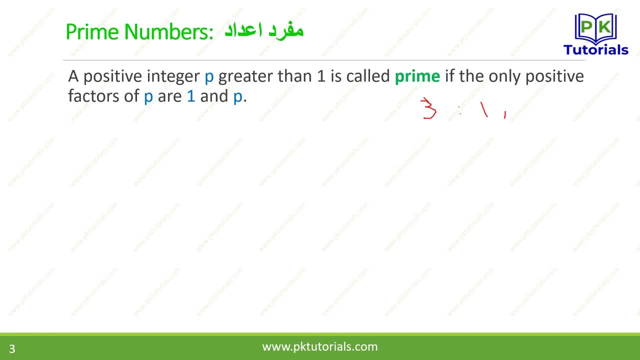 So by looking at this, it can be divided by 1 or by 3.. So here we have P and 1 and P, So P means the same number that we have taken. As we have taken P, so P means the same number, or 1.. 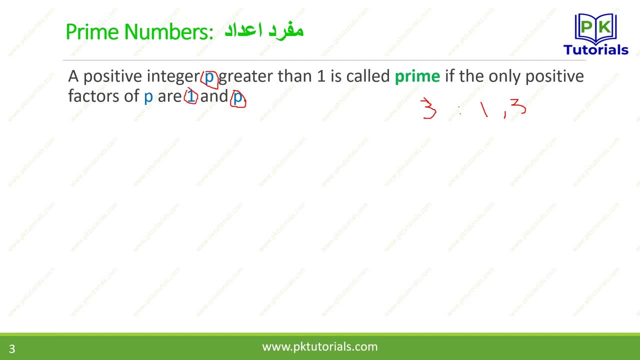 It can be divided by itself or by 1.. So we call this number Prime. Apart from this, it cannot be divided by any other number. Note that 1 is not Prime. So 1 is Prime. starts with 2. A positive integer. if any number is not Prime, then it is called Composite. 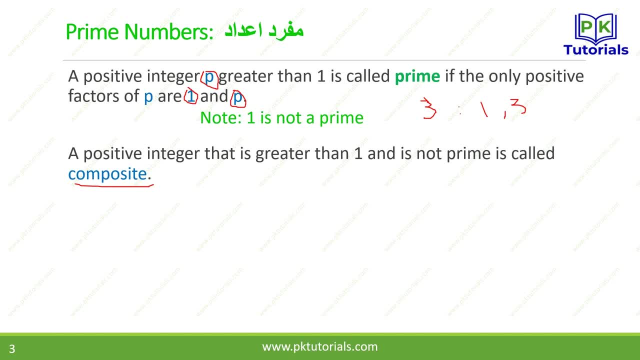 Then what do we call it Composite? So there are two types, either Prime or Composite. Pick any number, Either it is Prime or Composite. For example, now we have 4.. So what does 4 have? It is not Prime, it is Composite. 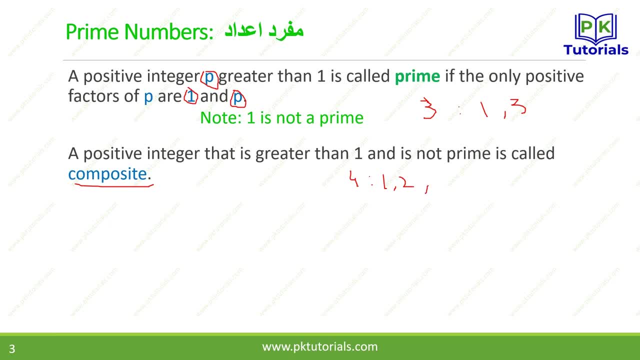 Because it is divided by 1,, 2 and 4.. So what is its factor? It is 3.. 1,, 2, 4.. So this is our Composite number, Fundamental theorem of arithmetic: In this every positive integer. 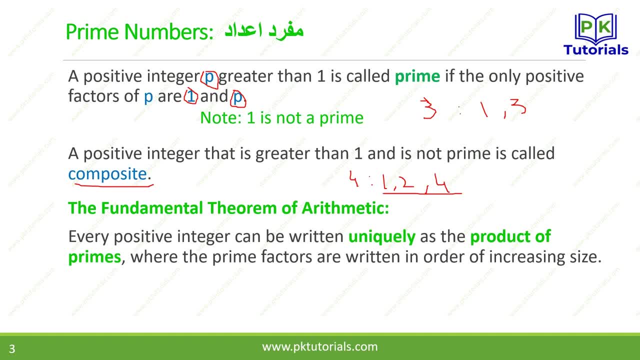 if any positive integer is taken can be written uniquely as the product of Prime. So we can write it as Product of Prime. It means where the prime factors are written in the order of increasing size. If any digit is taken, then we can take it as Prime. 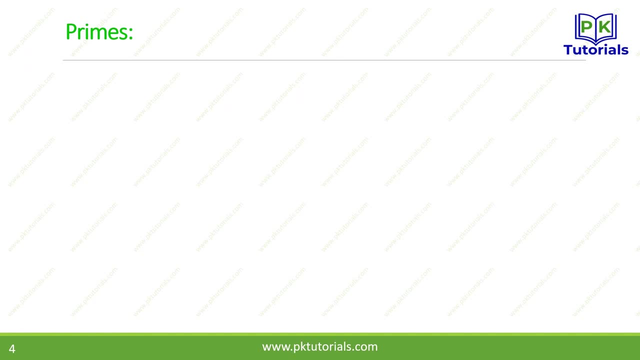 Let us see the example of this. This will help us understand. So the first example is 15.. Now 15 is a Composite number. In the theorem we have read that any integer, whether it is Prime or Composite, But the two factors of this number, 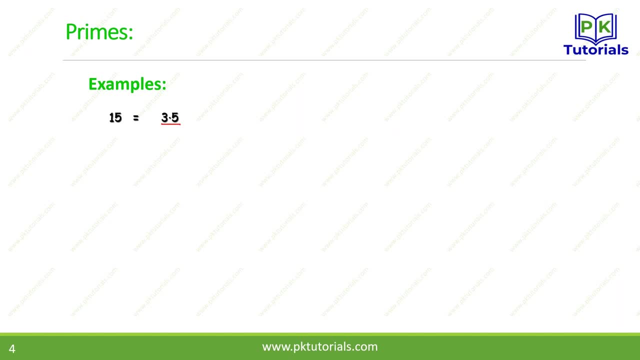 any two factors are 3 and 5.. Now, 3 is also Prime and 5 is also Prime, Similarly 48. So its prime factors are 2, 2,, 2,, 2 and 3.. So what do we have here? 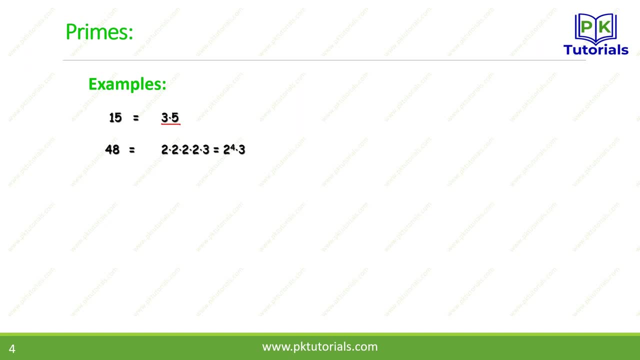 These are the Primes. Or we can write it as 2 power 4, 3. Similarly, 17.. Now if 17 is Prime, then it is 1 over 17.. Similarly, 100.. So we have 2 into 2, into 5, into 5.. 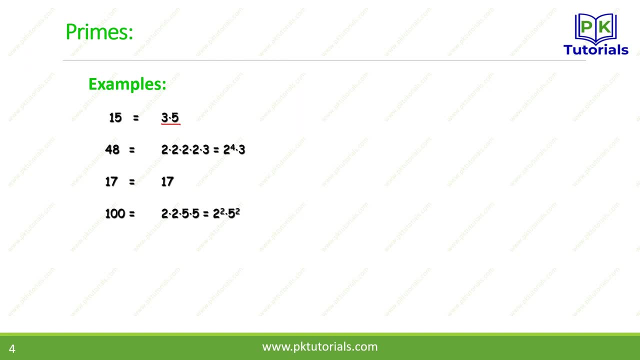 So 2 power 2 into 5 over 2 and 5 power 2.. So these are equal to 100.. Now 2, 2 and 5 are Prime numbers. So if any integer is taken then it will be the product of Prime. 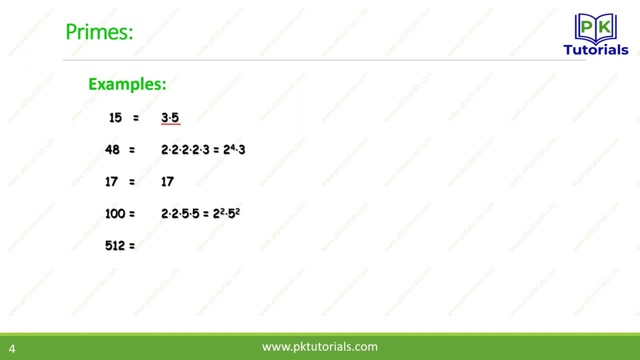 According to the theorem we have read, it will be Prime. Similarly, take 5, 1, 2.. So if you take this too, then multiply all 2 by 9.. So we get 512.. Similarly, take 5, 1, 5.. 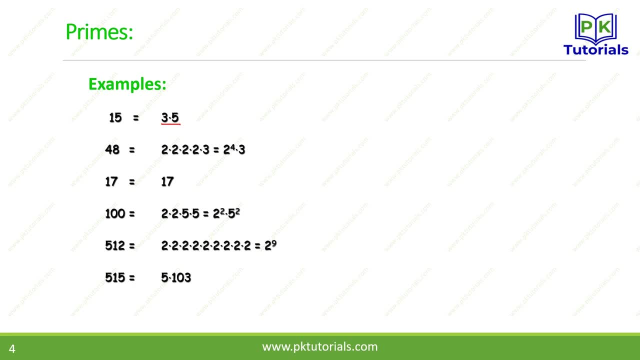 So this is 5 into 1, 0, 3.. Now what is 1, 0, 3?? This is also a Prime number. Take 28.. So 2 into 2 is 7.. We read again and again: 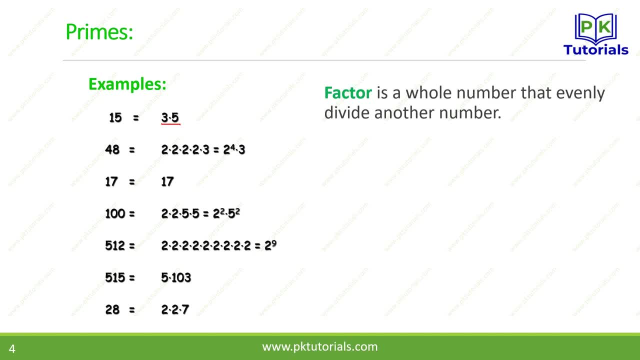 Factor or Multiples. So what is a Factor? What means by Factor? Factor is a whole number that evenly divides another number, That it evenly divides another number. For example, this is our 15.. So this is 3 over 5.. 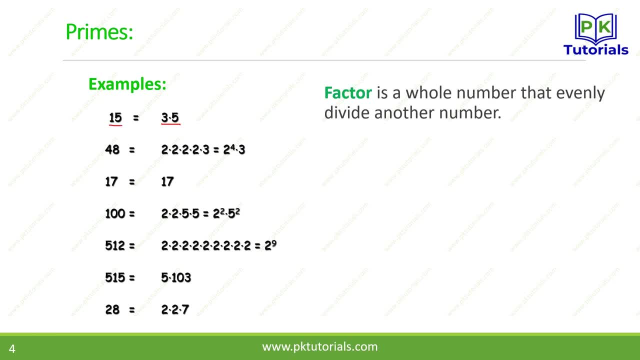 Now, 3 divides this by 5. And in this way, 5 also divides this by 15.. So what do we call this 2? Factor, Which is a whole number, So we do not take this as an integer in real value. 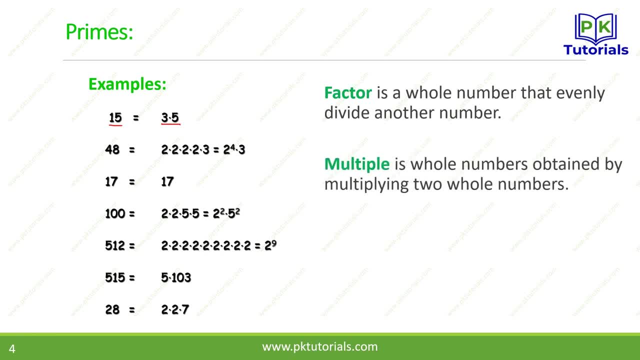 We take this as an integer, a whole number, And one is called multiple. So know the difference between Factor and multiple. What is the difference? in that Multiple is a whole number obtained by multiplying. So in this, what do we do? 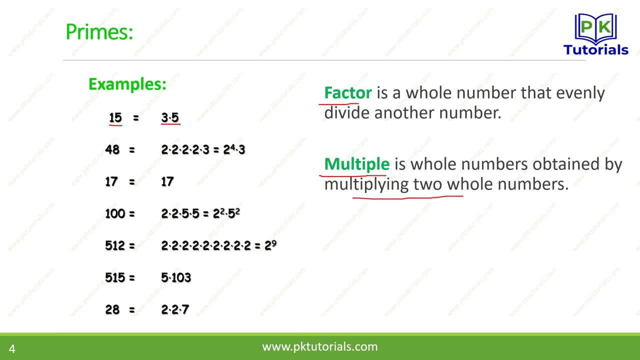 Multiply two whole numbers. In this we multiply two numbers, For example, if we take the first three multiples of 3.. So what will be the first three multiples of 3?? So 3 into 1,, 3 into 2,, 3 into 3.. 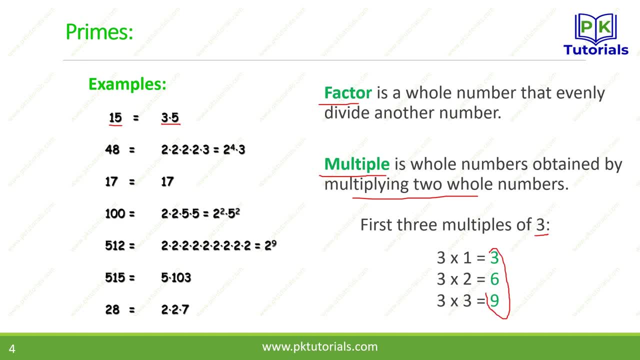 Now what will be the multiples of 3? 3,, 6,, 9.. These are the multiples of 3.. Similarly, 12,, 15, 18.. So these are the multiples. So the difference in this is Factor is the product of that number. 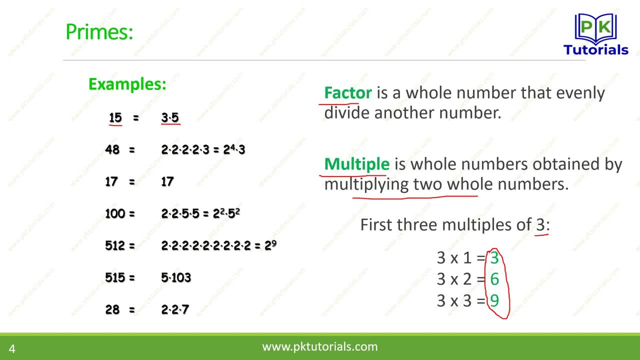 which is the prime number. We call it that. These are its factors which can divide it, And in this multiplication comes In multiple. With that, any number can be multiplied With 3, 1 can be multiplied With. 2 can be multiplied. 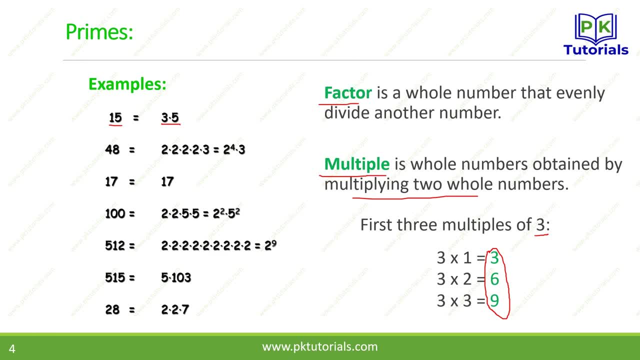 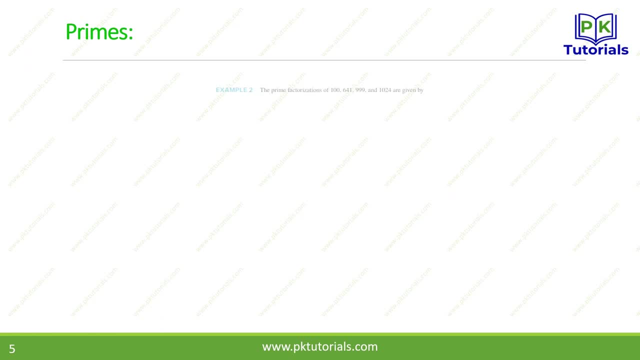 So we have multiples. So in this gap comes In this way: take 4,, take 5.. If you take 5, then 5,, 10,, 15,, 20.. So these are the multiples of 5.. 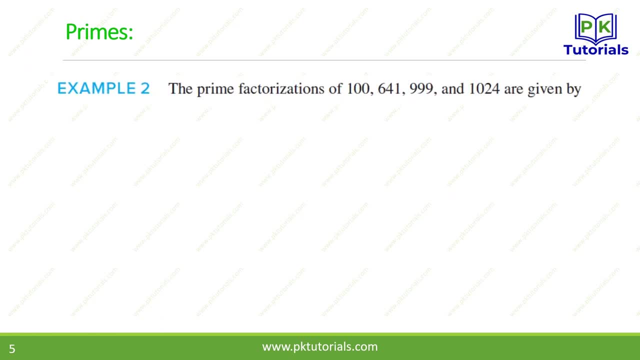 So prime is an example. How do we do prime factorization, Prime factorization of 100,, 6,, 41,, 19.. These can come with you, For example, in MCQs you can come to the question to do its prime factorization. 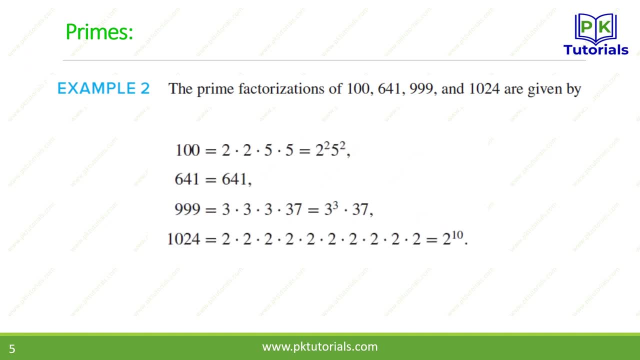 So 100 is 2 x 2 x 5 x 5.. So in this way you can write, or in this way in the shortcut: 2 power 2,, 5 power 2.. In this way you can write: 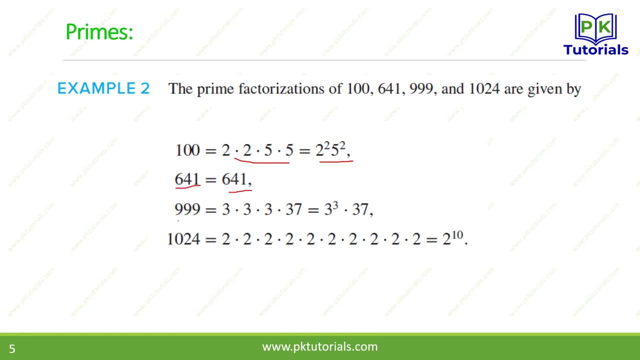 6,, 41, because it is a prime, so it comes with the same number. Similarly, take 999.. So in the end, 37,, which we have, is also a prime. So now divide it 1024.. 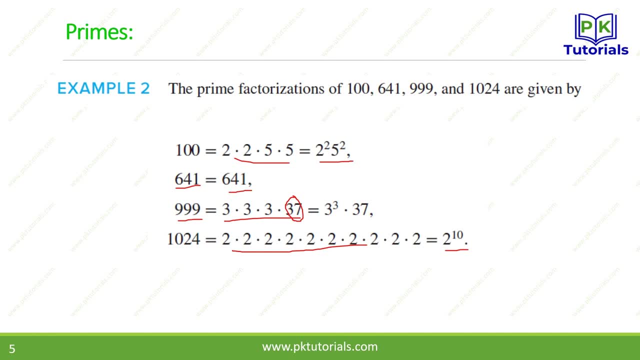 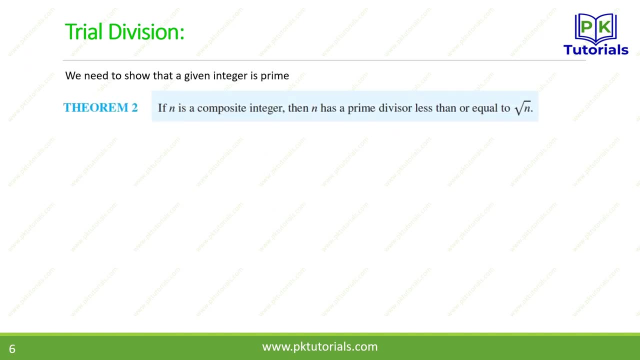 Now we have 2, power 10.. These are all its factors. Multiply 2 10 times, So next we have trial division. We need to show that given integer is prime. So the way we have taken prime, that we have a number, 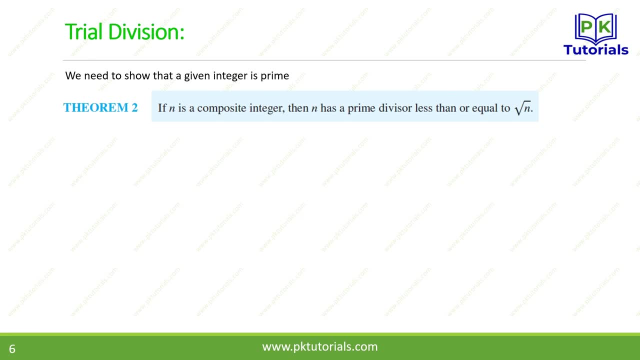 prime. how can we say that this integer is prime? So there is a theorem: If n is composite integer, if n is a composite integer, then n has a prime divisor, So its prime divisor is less than or equal to n under root. 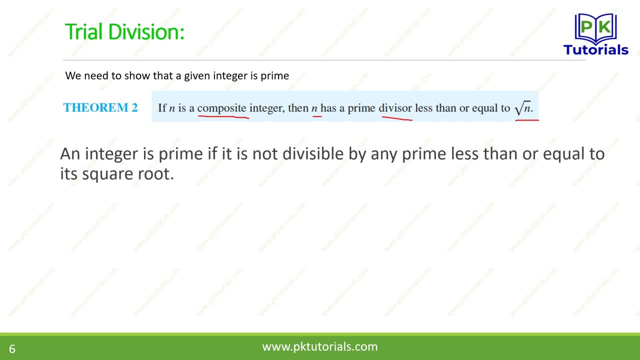 So its n under root will be less than that. An integer is prime if it is not divisible by any prime less than or equal to its square root. On the other hand, if we assume that any divisor will not be greater than or equal to, 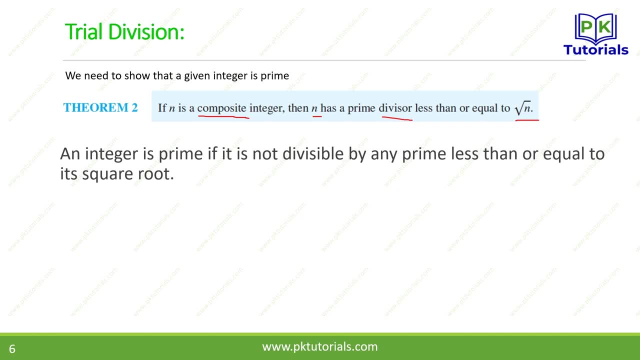 its square root, or will be equal to, or will be less than or equal to its square root. We consider this as an example. This leads to a brute force algorithm, known as trial, And what we have studied in this theorem is: what is a brute force algorithm? 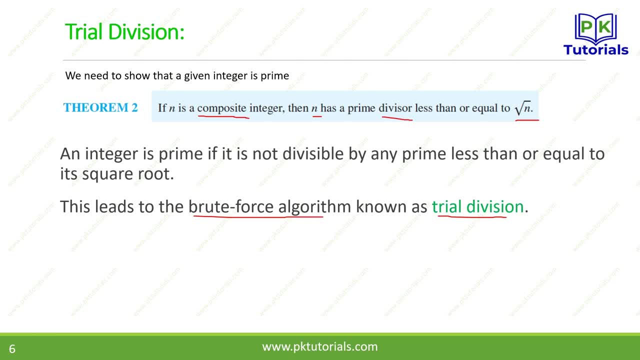 So what is a brute force algorithm? What is a brute force algorithm? You can try to find out what a brute force algorithm is. You can read a brute force algorithm in another course in Data Structure. So this algorithm is that you can try whatever is less than 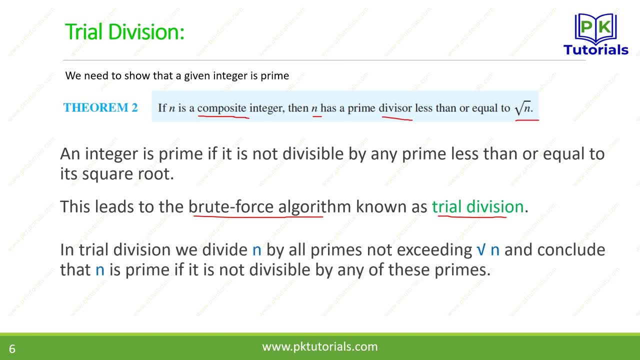 or equal to its square root. In trial division we divide. What do we do in trial division? We divide n by all primes, not exceeding So. all primes means. this is a brute force that first check 1, then 2,, then 3,. 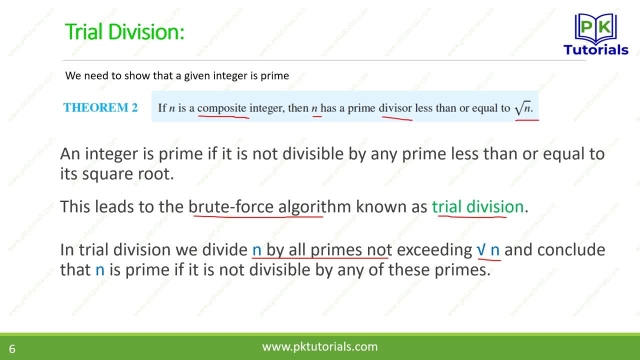 then n. So all primes you have to check, but not exceeding under n under root. So it will not exceed under n under root. So we take an example of this trial division. This is the theorem we have. It is easy if n is composite. 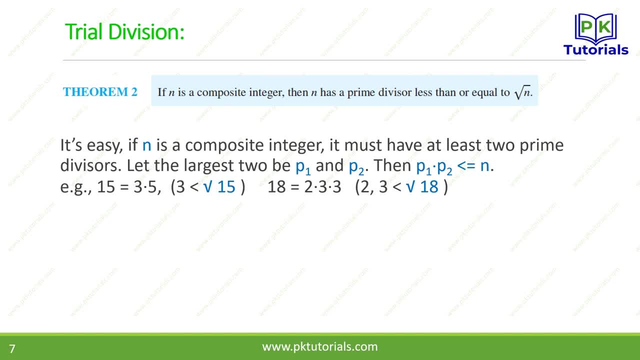 because it said that n is composite, it must have at least two prime divisors. We read that it must have at least two prime divisors, p1, p2, then p1 into p2 is less than or equal to n, For example. 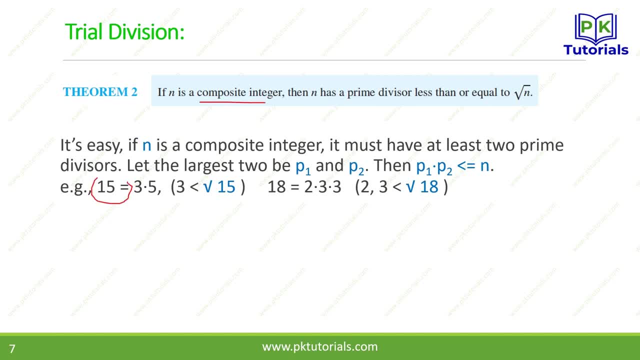 we have taken 15.. Now what is 15?? We have a composite number or composite integer. So its two prime factor is 3 and 5.. Now take 3. it said n has a prime. a means at least one prime will be. 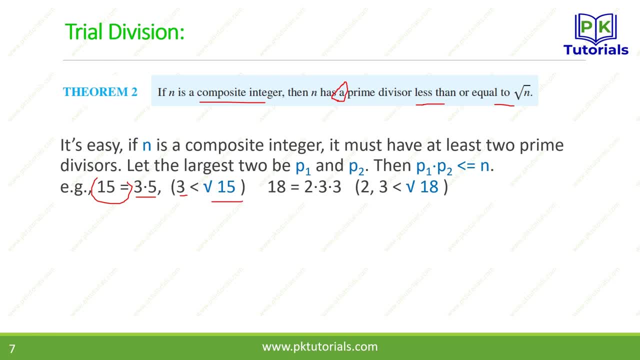 less than or equal 15 under root. here is n under root, so if this is 16, then 4 will be approximately 3.8, or something like this: Check this: 4.. So this will be bigger than 3, which means that 3. 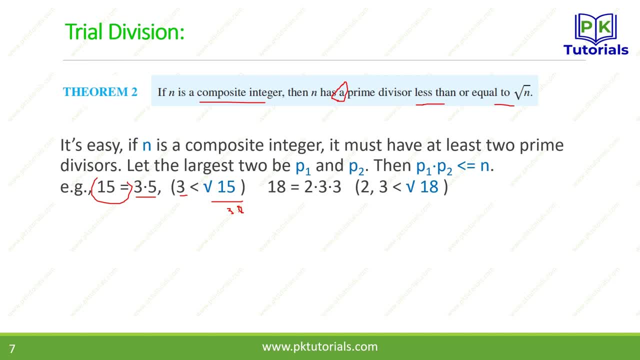 will be less than 15 under root. So this factor 3 is less than this 3.. Now look at 2.. 2 is less than 18 under root. So it said 1 will be less than 1.. It can be. 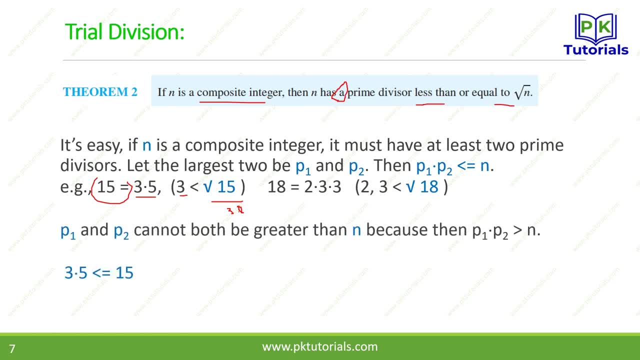 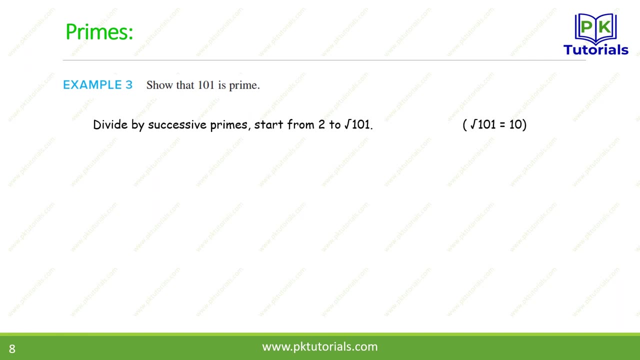 2 or 3.. So p1 or p2 cannot be greater than n And this is greater than n. We have taken the meaning of the number of digits. Now we have to prove that 101 is prime according to trial division divided. 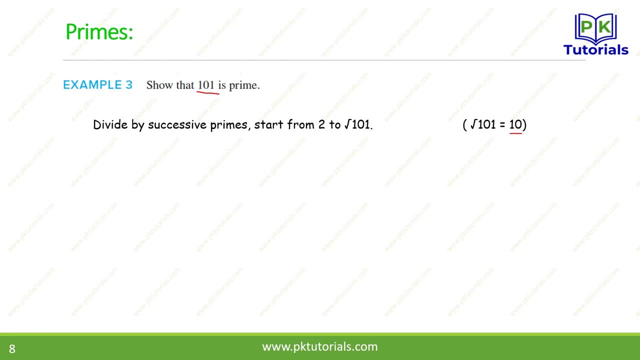 by successive primes Start from 2 to 101.. Now if we take 101, 10 and divide it by the prime number, So the only prime not exceeding 101 are 2,3,5,7.. Less than 10 is. 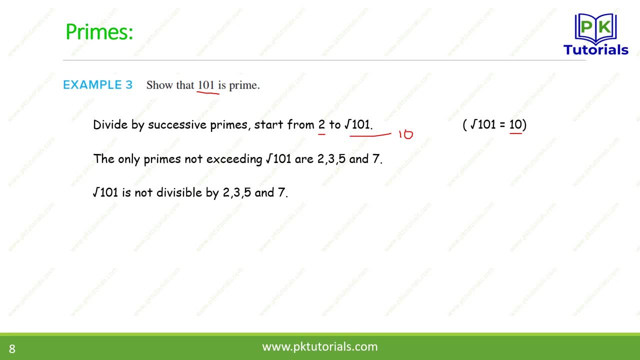 prime and we have 2,3,5,7.. Now we divide this by 1.. So 101 is not divisible by 2. It is not divisible on 2,3,5.. Now we have another example. Find the prime. 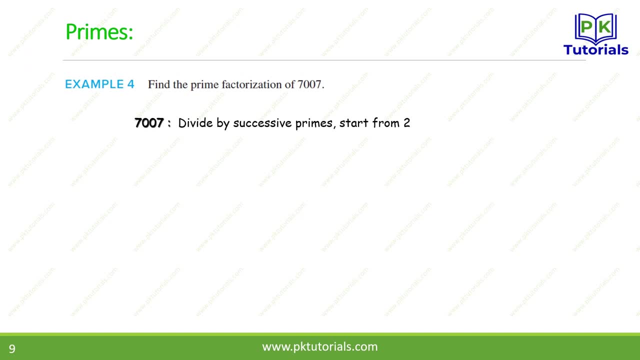 factorization of 7007.. We have to do prime factorization of 7007.. So first we take 7007 and start from 2. Because first prime number is 2. Then prime is not divisible on 2 and 3.. 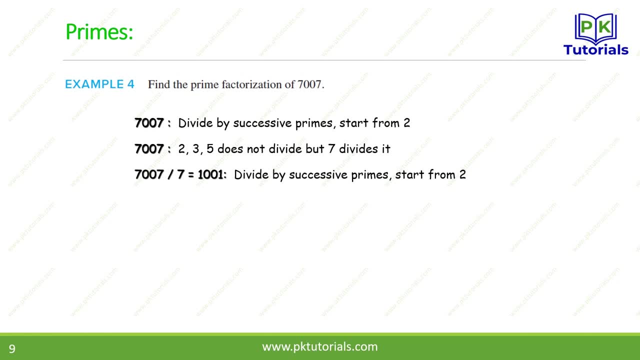 Why? Because if we divide this by 7, we get 1001.. Now we take 1001 and divide it by 2.. Now look at 101.. We see that it is not divided on 2,, 3,, 5,. 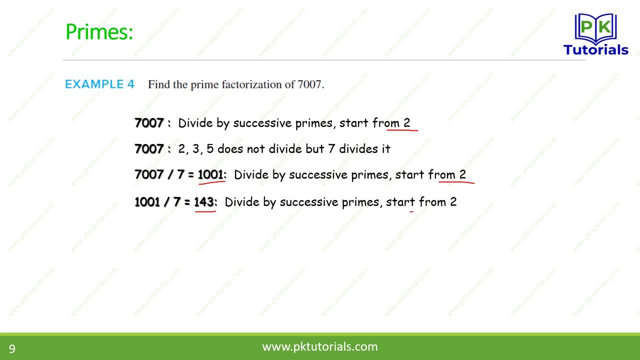 Now start. 1,, 4,, 3 from 2.. This is divided by 2,, not by 3,, not by 7,. 5,, 7, 11.. This is divided by 11,, so we have 13.. 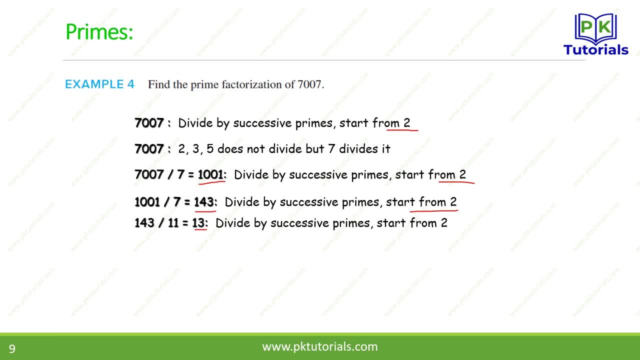 Now, if we divide 13 by 2,, then it is not divided by 2, but by 3,, 5,, 7,, 11, and 13.. So now we have the lowest number, which is not further divided. 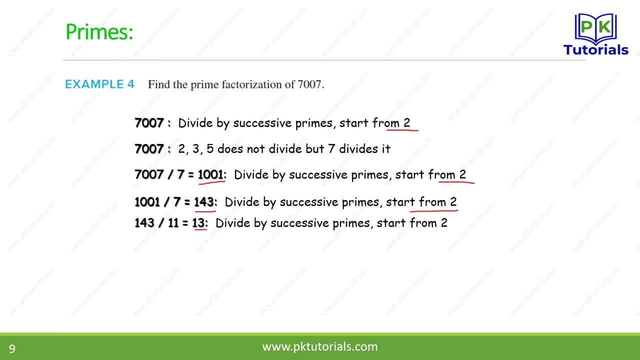 When you have the last prime number here, because it is not further divided, then it stops. Now what we have to do is whatever we have divided. first it was 7,, then it was 7,, then it was 11, and then it was 13.. 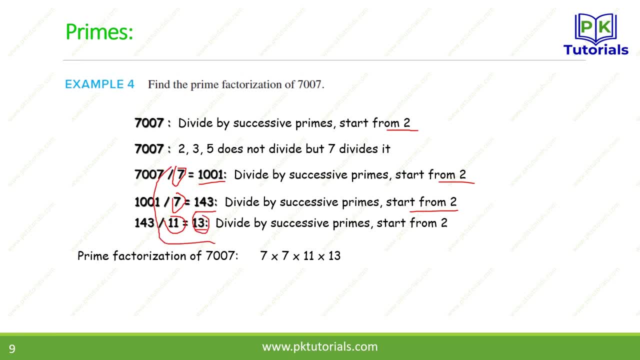 So you multiply all of these by this And what we call these. these are its prime factors. Now, if you multiply all of these, then you will get the answer 7.. 7, 0, 0, 7 will come. 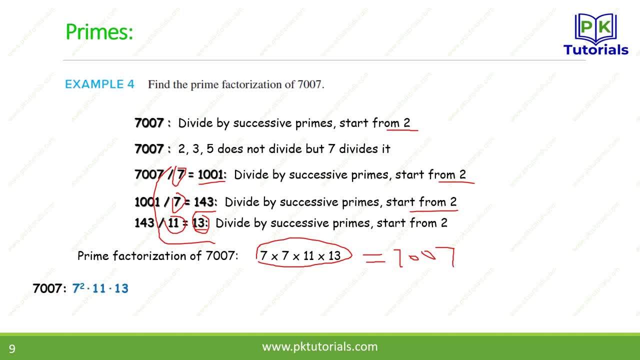 The same number has gone. So these are all its prime factorizations. Okay, you can write it like this: 7 squared into 11, into 13.. So we call this method, this trial method, revision method. we have done its prime factorization. 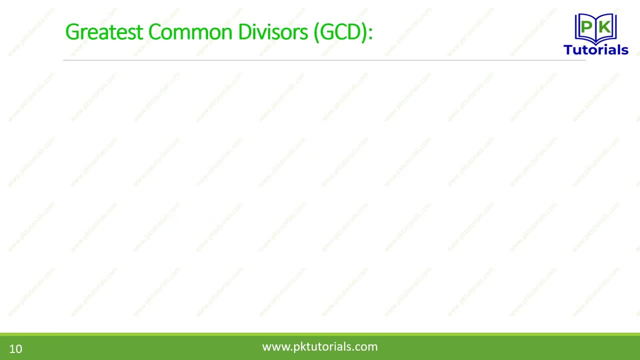 So next we have GCD, or Greatest Common Divisor. Till now, what we have said, what were all the divisors, that is that Now we have GCD, or Greatest Common Divisor. Now we look at Diversor GCD. 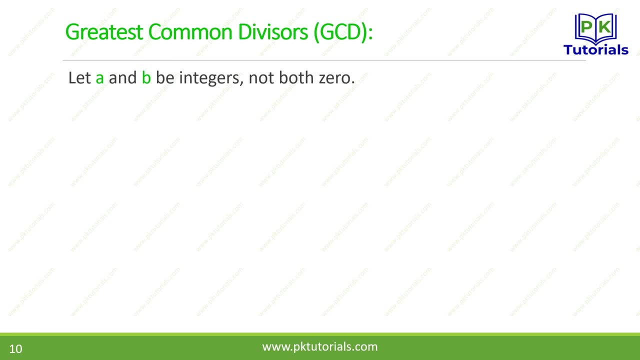 If we have two integers and if there is no zero in it- A or B- So what we call the Largest Integer, D. Now we have taken another number, D. What it does? it divides A and divides B. 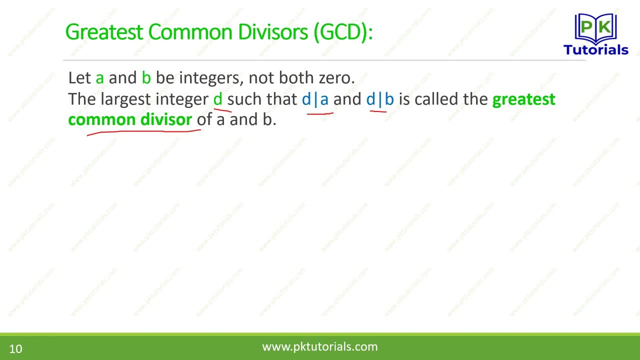 And we call this that we have Greatest Common Divisor, both for A and B. But we cannot think that the D will be the Largest. it can be smaller than this as well. So the greatest common divisor of A and B is denoted by GCD of A and B, because it is the greatest common divisor of both integers. 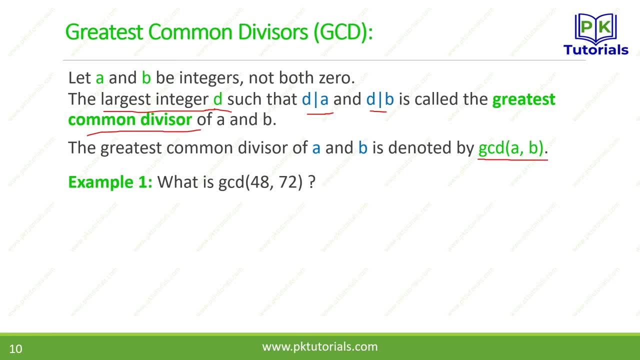 Example: what is GCD of 48, 72?? For example, we have 48 as A and B, So what will be the GCD of both integers? First, we have the positive common divisor of 48 and 72.. 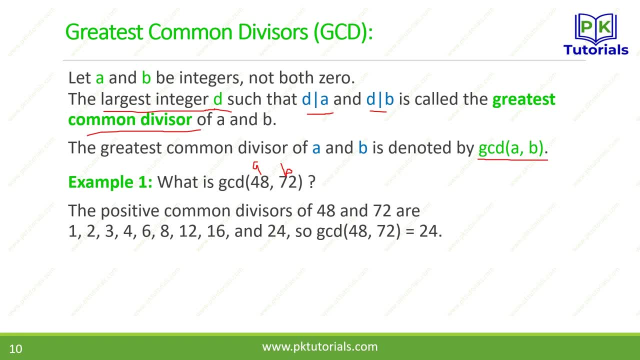 We know all the prime divisors of both integers, Then we divide the common divisor of both integers equally. So we have 24 GCD of both integers, because A can also be divided by 40.. So we have 24 GCD of both integers, because A can also be divided by 40.. 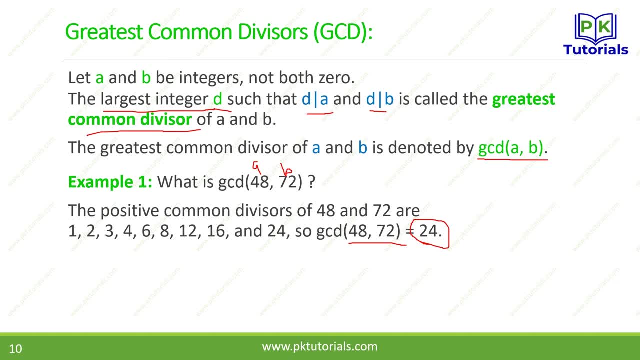 Similarly, we have 48 of two integers and GCD of 42.. Similarly, we have 48 and 38, so we need to divide these two lengths equally and multiply these two by two. Similarly, we have 48 and 38, so we need to divide these two lengths equally and multiply these two lengths equally and multiply these two lengths equally. 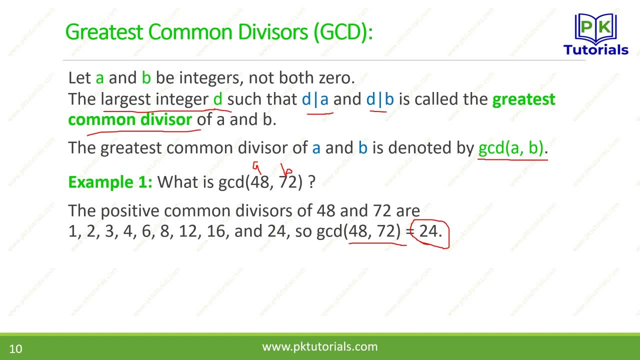 So sweetheart can also be divided by 2 and gives us 46. However, we do not have sector factor and GCD of both integers. Therefore, most common divisors of these integers are two. GCD of both integers is one. even GCD of both integers is equal to a. 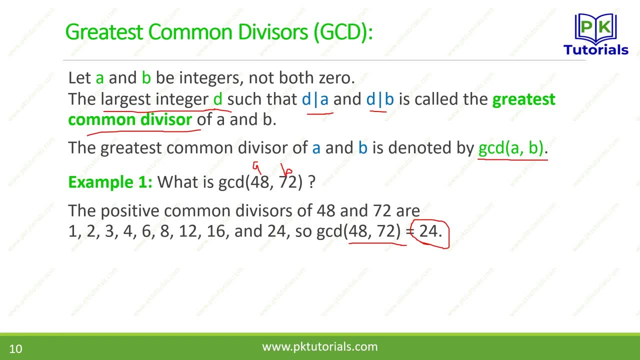 in follow, known as GCD of both integers. It should be known that two and GCD of both integers is equal to a. It belongs to the same family of GCD. Similarly, we have an equation of 2 with 19 and 2 with 72.. 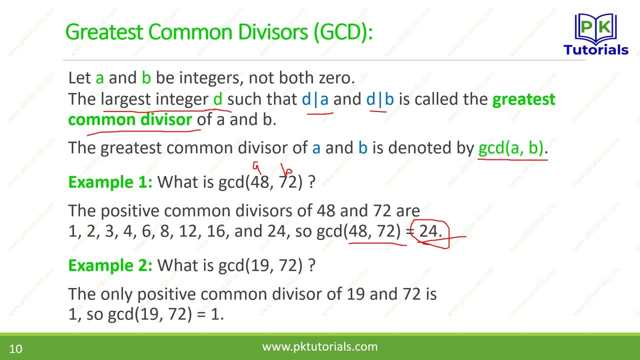 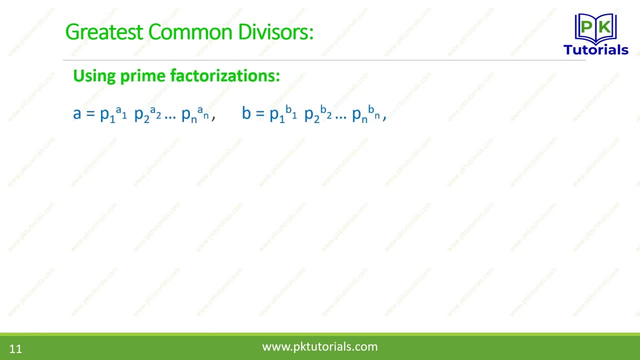 The你说ator repeating the formula: Only positive common divisor is O1, because no one can divide it like this. So we say that O1 is the common divisor and that is its GCD. After this, using prime factorization. Now the prime factorization that we have just read, that if we take a number and take its prime factor, as we did in the last slide, 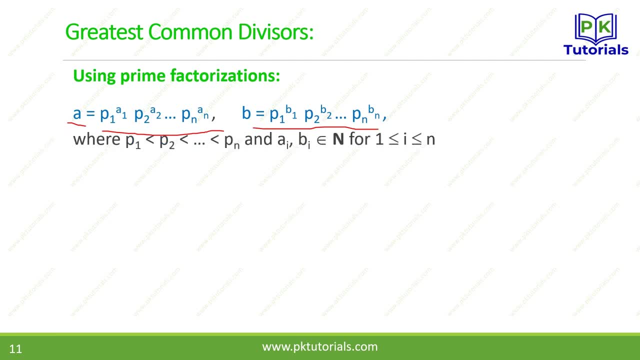 take the prime factor of both, where P1 is less than P2 and we can write it in increasing size. So the GCD that will be in P1, P2 up to Pn, the minimum that will be in their power, we say that it is their GCD if we multiply it. 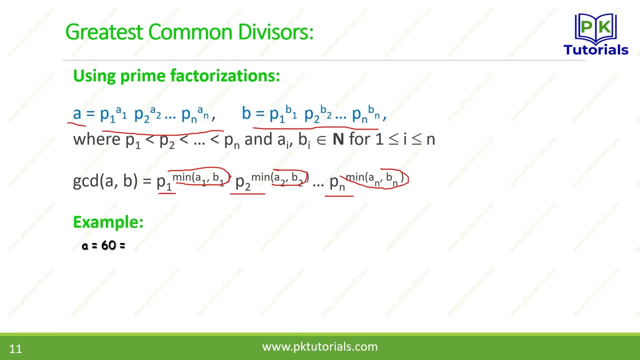 How do we do this with an example? For example, there is an integer A. This A is our GCD. We have 60.. So the prime factor of 60 is 2 power 2, 3 power 1, 5 power 1.. 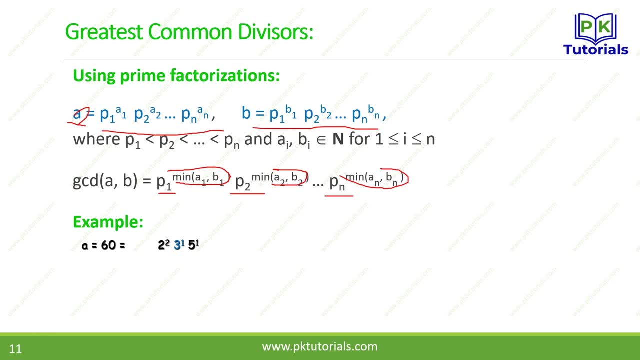 Because it is one time and 2 is two times. Multiply 2 into 2, into 3, into 5.. So we take its power. There is no need to write 1 on the one time, But for you to understand that we should write 1 on it, 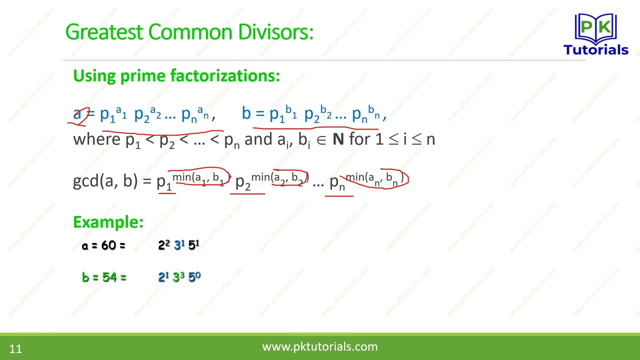 Similarly, we have 54 as B. Now the prime factor of this is 2, 3 into 3, 3 power 3 and 5 power 0. Now see where you have 2, because it should be the same. 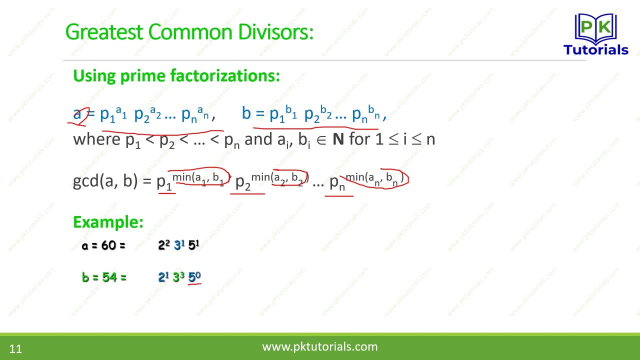 If there is no one, then you have 5 power 0. Because its value is 1.. If you have 2 at any time, then you say that we cannot get the same value of both. So what you have to do is take the power 0 of the one that is present and not present in the other. 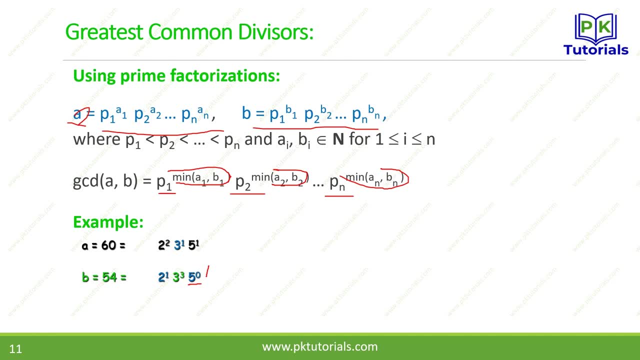 Because with any number 1 is multiplied as much as you want, That number comes. So here we do not have 5 power 0. But it is their prime factor, So you can write 5 power 0.. 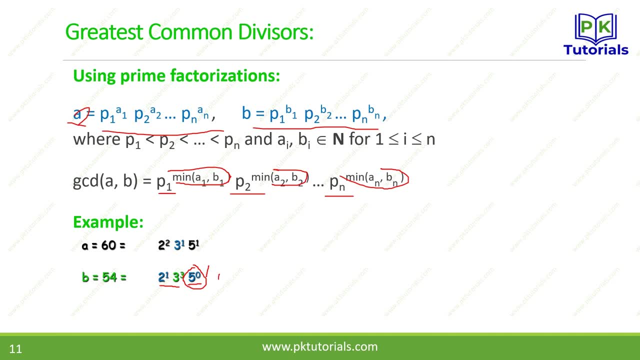 Because it is equal to 1.. So you can multiply it. Now what we have to do? We have said that the minimum of A1 and B1.. We have taken the minimum of both of them. Now this is 2 power 2, and above it is 2 power 0.. 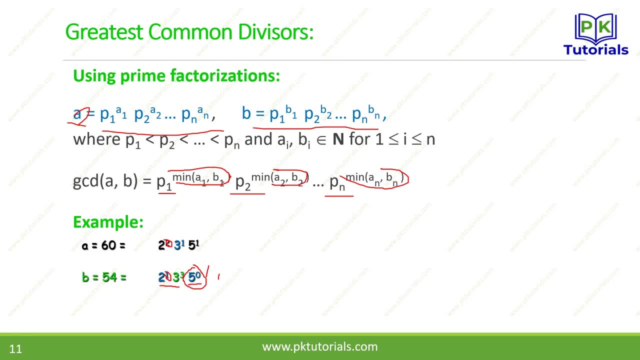 Their base should be 1.. So the minimum of both of them, What is the minimum We have? 1.. So we have taken 2 power 1.. After this, clean it. We have taken this From here: 2 power 1.. 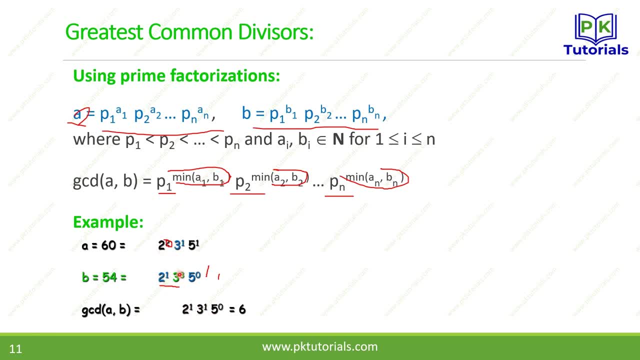 From here we have taken this blue. After this: 3 power 1 and 3 power 3.. So we have to take the minimum of 1.. Similarly, 5 power 1 and 5 power 0. So we have to take the minimum of 0 and the minimum of 0 out of 1.. 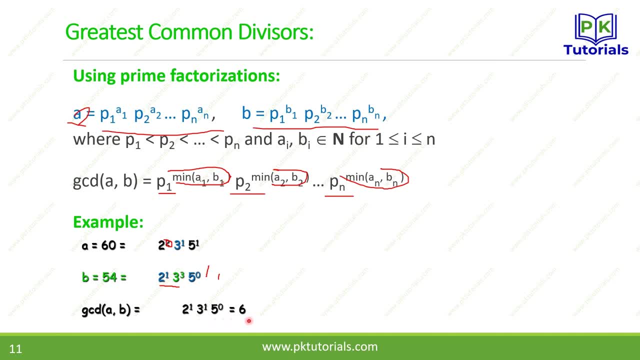 So we have GCD 2 into 3 into 5, power 0. So we have 6.. Now 6 divides both A and B, So we say that this will be its greatest common divisor. Next, we have relative prime integers. 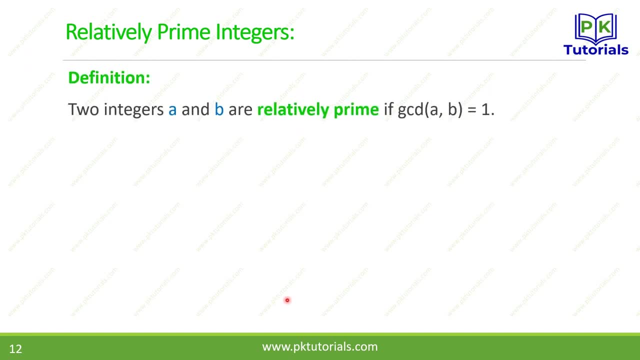 What are relative prime integers, Two integers: If we have two integers, A and B are relative prime if GCD of A, B is equal to 0. If in these, as we gave one example last day of 19 and 72, its GCD was 1.. 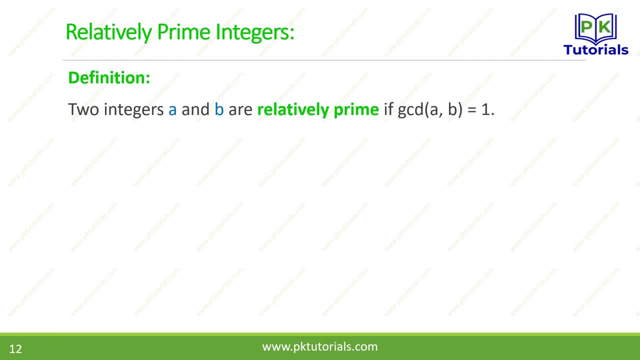 If any of the two integers have relative GCD 1,, that is, any common greatest divisor in it, then we can say that they are relative prime. Example 15 and 28,. are they relative prime or not? You can see whether they are relative prime or not. 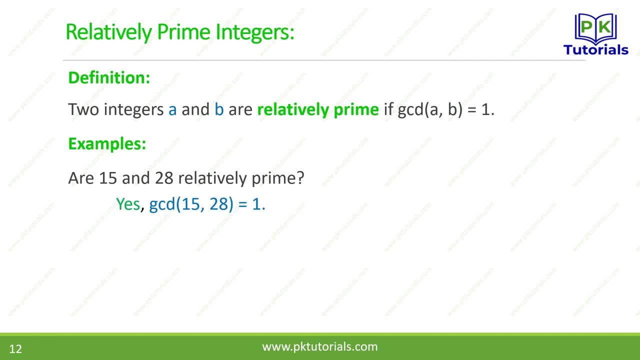 Yes, because 15 and 28 are relative prime- See 15- and 3 and 5 are relative prime, So we have 3 and 5 as its divisors. Similarly, we have 2 and 5 as its divisors. 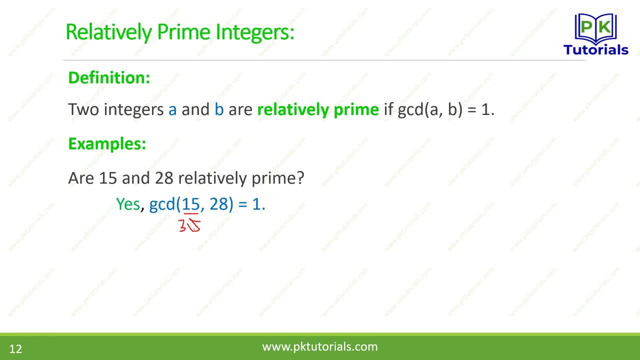 Similarly, we have 2 and 5 as its divisors. So you have 2 and 5 as its divisors. Similarly, you also have 2 and 7 as its divisors. Similarly, you also have 2 and 5 as its divisors. 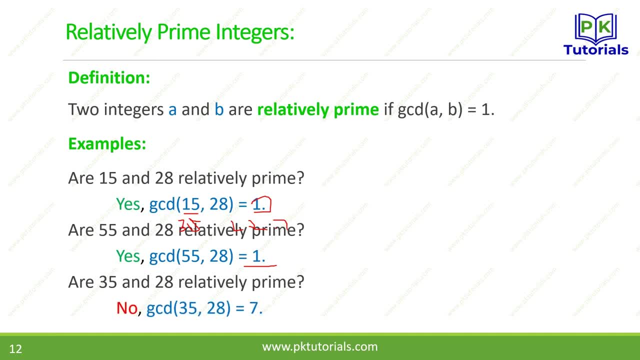 and 7 as its divisors. Similarly, we have 5 and 7 as our divisors. So we know that 2 and 7 is quite big. But right kiya hai 7, ata hai 7 into 5, 35, 7 into 4. hamare paas 28 to ye. hamare paas gcd 7 hai to ye. 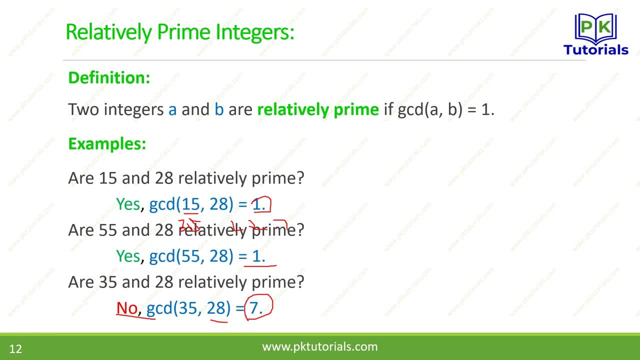 so we can't say say that they are not relative prime o sirf only jo first: 2 hai hamare paas, ye 15, aur 28, 55 ye hamare paas relative prime hai aapas mein. so is ke baad hai pair wise. 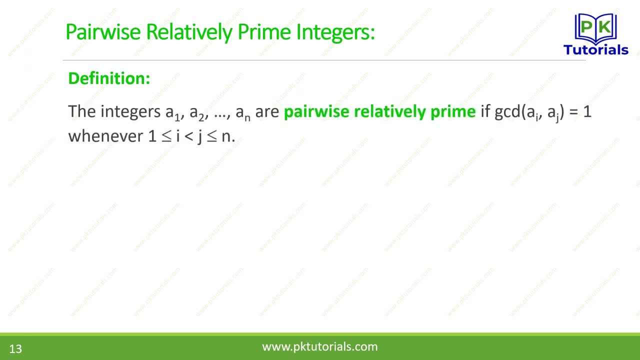 relative prime todasa. aur add karte hai, agar hamare paas jo abhi hamne 2 ka, kya agar 2 se zyada ho, to ham usko kehte ke pair wise yedi: a1, a2 upto a n if gcd of a, i, a, j. 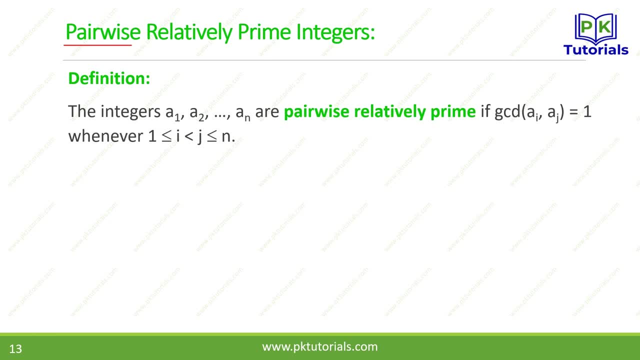 a, i aur j ko ham 1 upto n karte hai yeni 2 se zyada value ho 3, 4, 5, to usko ham kehte pair wise relative prime. so ye hote ke relative mein sirf 2, the pair wise mein hamare paas. 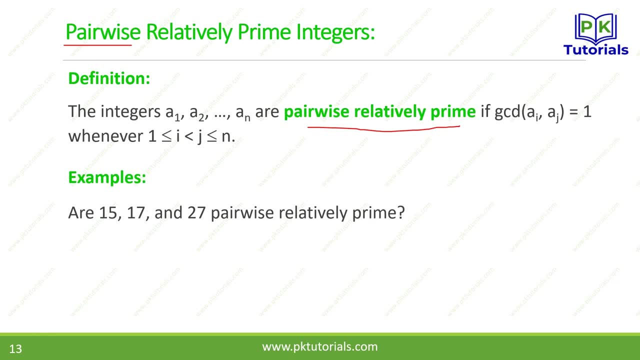 pairs ho gayi. yeni 3 ka pair ho gayi. ye dekhe hamare paas 15, 17, 27 pair wise relative prime. no kyunke sab ka jo gcd hai, so we can't say that they are not relative prime. o aapke paas 1 hona chahiye. ab is mese jo aapko samayne ho. ye hai ke kui bhi 2 value. 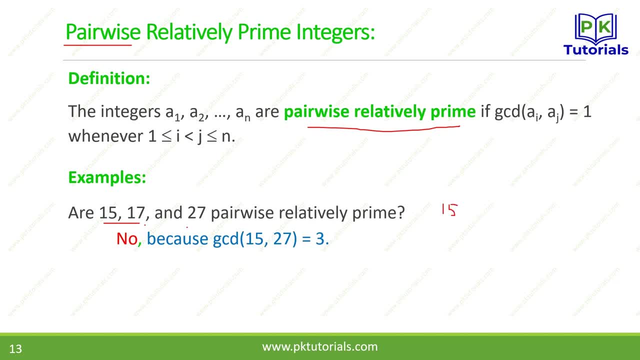 utaade 15 kyunke 3 value hai hamare paas 15 aur 17, ab is ka 15 aur 17 ka jo gcd hai hamare paas is ka jo gcd hai o to hamare paas 1 hai isi tara 15, 17 aur 17 kui bhi kyunke idhar. 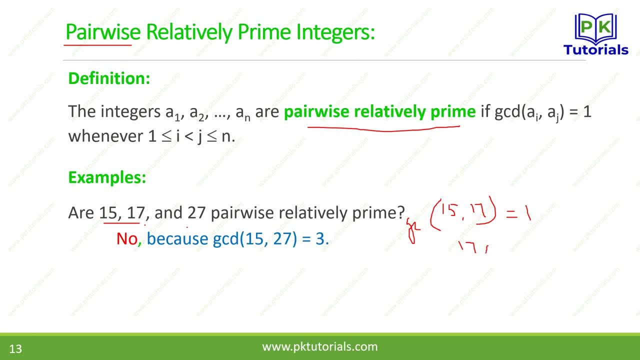 a aur i aur jai, kui bhi aapke paas 1 ho na chahiye. ab is me, se jo aapko samayne ho, ki aap number le sakte, 17 aur 27 is ka. agar aap gcd le le, to o bhi 1 hai, but jab aapne 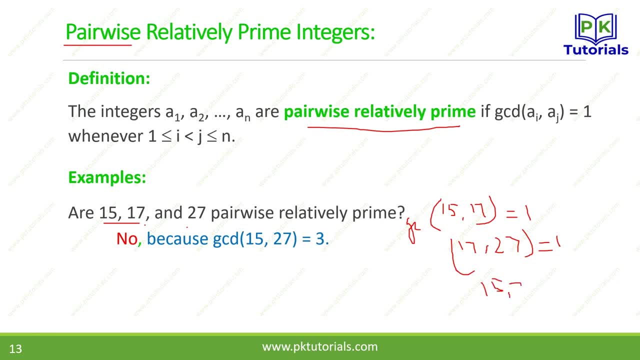 15 aur 27 ka liya. uska jo gcd hai hamare paas 15 aur 27 ka o hamare paas 1 nahi hai o kya hai? hamare paas 3 hai, kyunke 3- 15 ku bhi divide krta hai 3 into 5- 15 aur 3, 28 ku bhi. 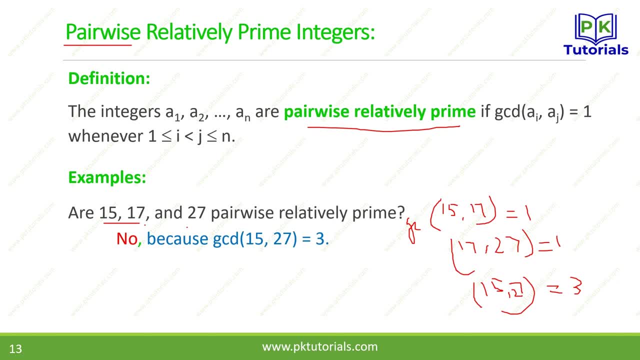 krta hai, 9 into 3, 27, toh lehaza, they are not relative prime. so they are not relative prime. toh is te me, se aap ne ye check karna hai, ki wo saray pair 2, 2 ku uta ke check karna hai. 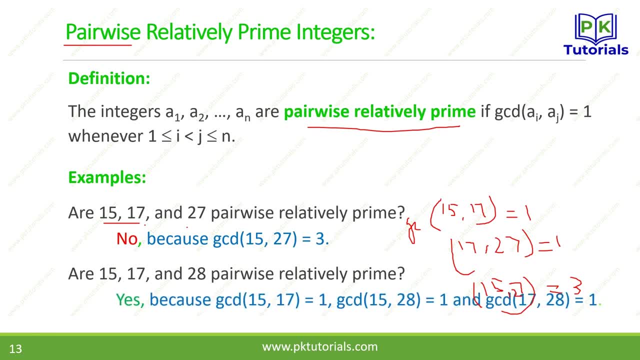 isi tara 15, 17, 28 ye dekke. yes, ye hai kyunke ab jo hamare paas jo third, aa ye 1 hai, gcd 1, 17 aur a ye jo last 28 hai. is ka bhi 1 ahta hai. ab dek hai samayne hamare paas saray. 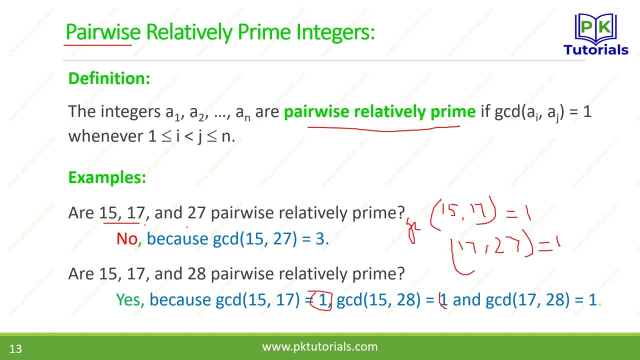 sab ka kya atha hai? 1 ata hai. idhar bhi 1 ahta hai. each side also 1 atha. haiيدhar bhi 1 atha ho fahi beads. Now we have relative prime, pairwise relative prime, all three of them together. 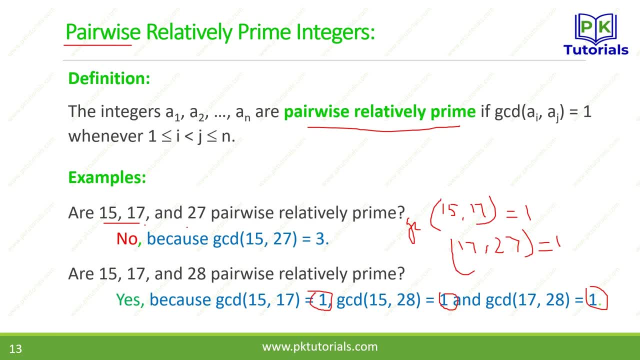 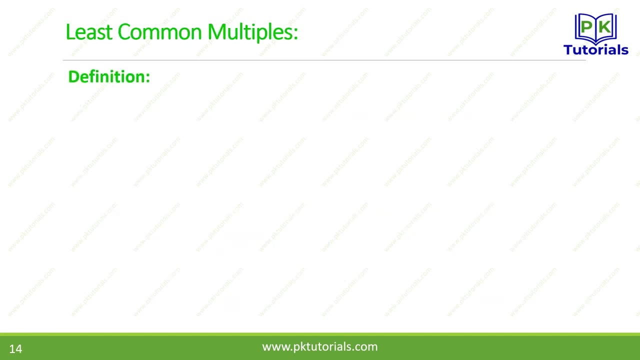 Now it is not necessary that any number in this like 28,. now you say that its prime is not necessary, it is any composite integer, but its GCD should be 1.. After this list common multiple, or what we call LCM. so list common multiple of the positive integer A and B is the smallest positive that is divisible by both A and B. 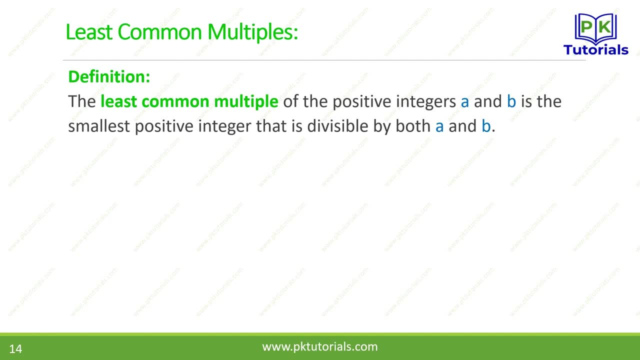 First in GCD we were looking at greatest. in this we will look at least smallest positive integer. so we write it: LCM, ie LCM of A or B or small or capital, we write both. So this is an example now. LCM of 3, 7, we have 21,. now in the last we read greatest common divisor and here we have multiple. just like we defined multiple in the last, that multiple of 3, which we have is 6, 3, 6, 9, so in this you have to multiply both of them together and take the smallest number from that which divides it. 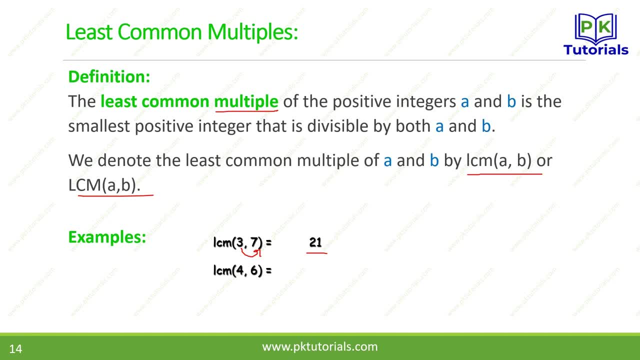 Similarly 4 over 6, so in 4 over 6, we have 12,. ok, now see in this also, if you multiply these two, we have 24, but it is not the least that can be divided over these two, ok. 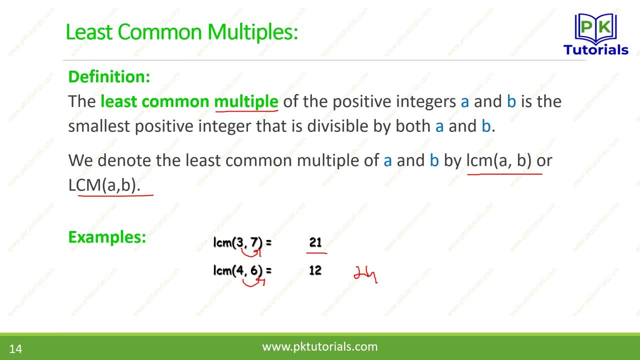 So this is one method that you multiply both of them together, but it is not necessarily that it is LCM of that. ok, this is the situation, because there is no lower value than this, that it can be divided over 3 or 7.. 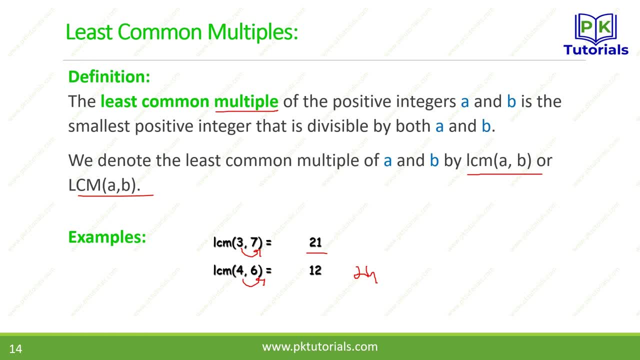 Because in this we have 12 divided by 4 and 6 on it, because it is a multiple of the list. 3x4 is 12 and 6x2 is 12, so this is the multiple of both of them. so how many can be the multiple of this? if you do 4, then it is 12 and 4 is also 12, like this, and 18 is also 6, but the list will be the most common among all of them. 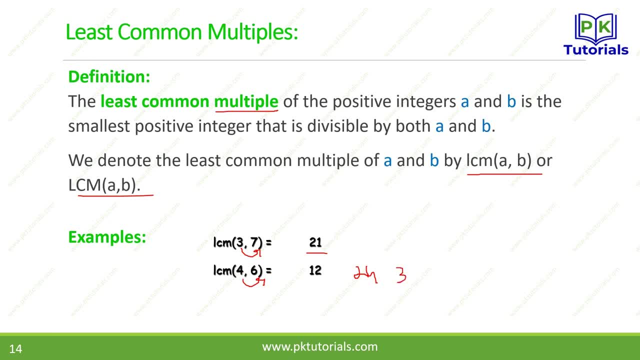 The second one is 24 and after that we have 36, which is the most common, and after that we have 48, but the smallest one we have is 12 and we call it LCM, list common multiple. Similarly, we have 10 for 5 and 10 and apart from that we have 15, 20, 30, 40, but that is not LCM. the least common one is not the smallest one, and if we take the smallest one, then we have 10.. 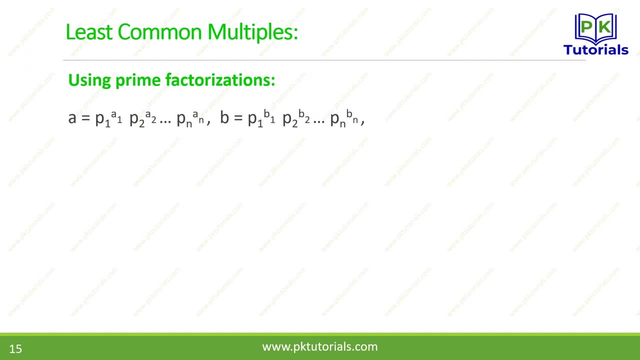 So using prime factorization is the same way as we did in last GCD, that we first make the factor of A and B. Now the difference is that in that we took the minimum when we were taking it from the power of GCD. so in LCM we have to take the maximum. 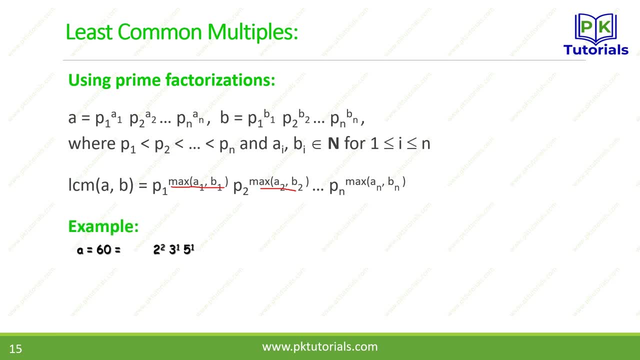 For example, the same example which we took last. so 2 power 2 is 60 and we have 50 for A and B. Now, in the last we took 2 power 1 because 1 was the least minimum. Now in this we will take 2, we will take 2 square and after that 3 in the upper one and in the lower one, 3 power 3 is the most common. 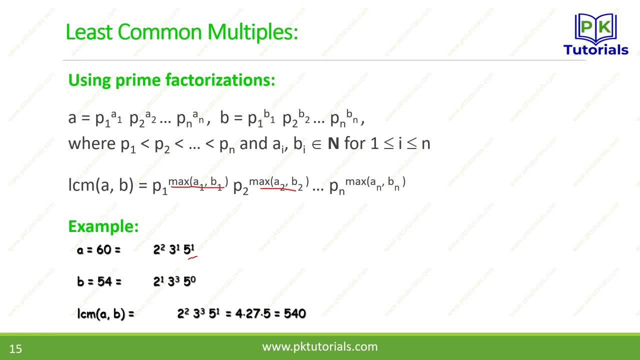 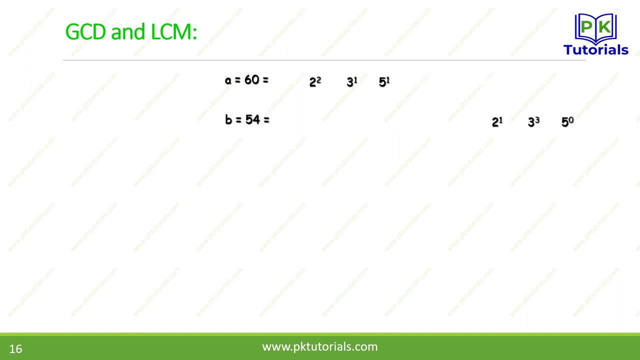 5,, 0 and 1, so in this 1 is the least common. so we take these three and we multiply it, so we have 540, which is LCM. Now let's see both of them together, GCD and LCM, which we took both in the same example, in GCD and LCM. 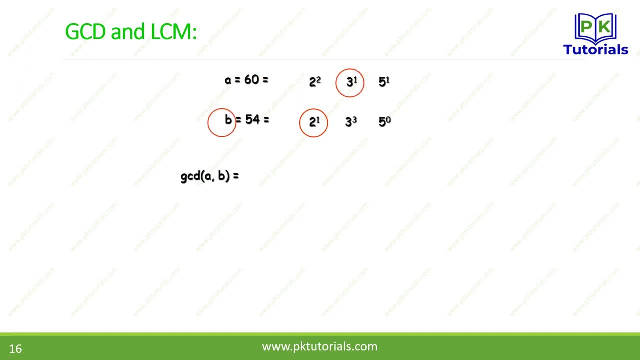 So in GCD we used to get the least, which we just pointed out, and we used to get 6 from its multiplication. In the same way, we took the LCM, which I circle in green, and we took these three. Now we have 540. 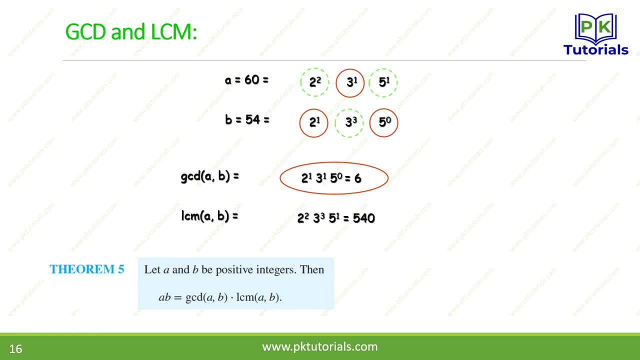 Now there is a theorem: Let A and B be positive integer, then A into B is equal to GCD of AB into LCM of AB. If we multiply both numbers together, A and B, then they will be equal to N multiplied by GCD, multiplied by LCM. 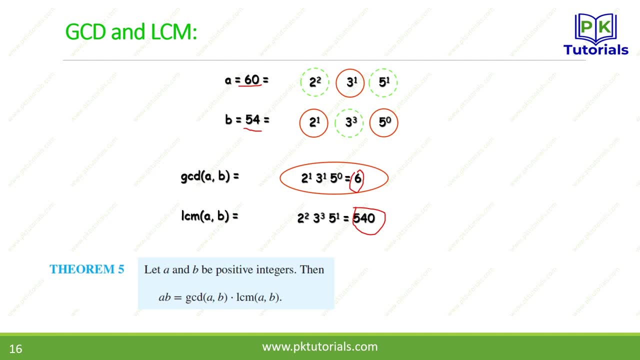 If we multiply LCM and GCD together, then they will be equal to N. Both numbers are equal in multiplication. How See this Now? we have: first number is 60 and second number is 54. Multiply these two together and we multiply 6 and 540 on the right hand side. 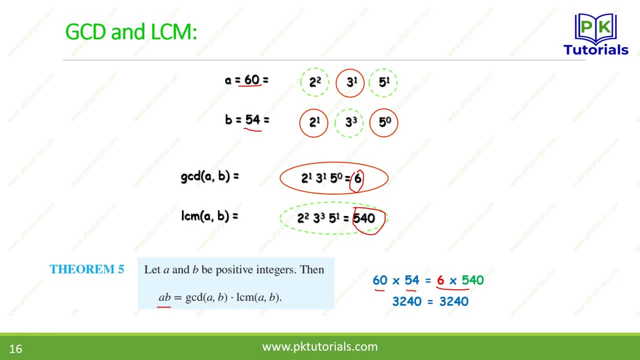 So on both sides we have 3,, 2,, 4,, 0.. Ok, So with this you can conclude this theorem. If you don't know a number, or if you don't know its GCD, then you can calculate it easily. 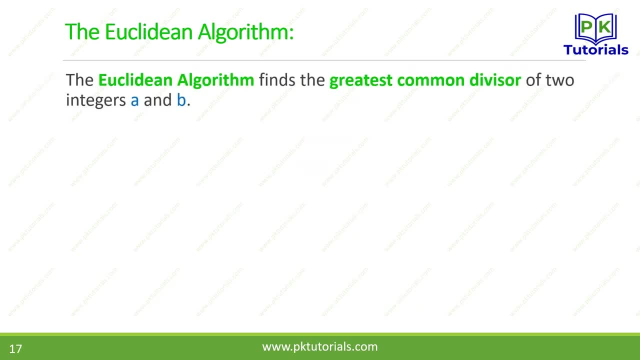 After this, we have Euclidean algorithm. With Euclidean algorithm, we find out the greatest common divisor of two integers, A and B. For example, we have 287 and 91. We have to find out its GCD. So what do we do? 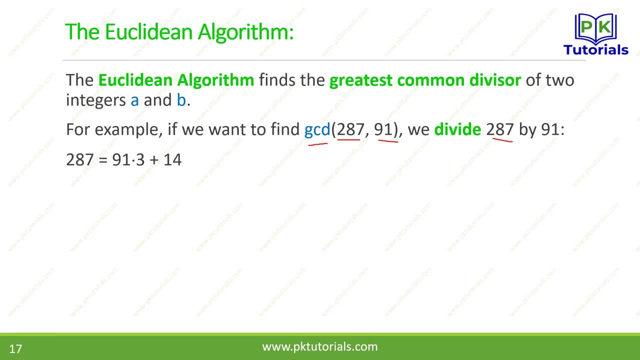 We divide 287 by 91. So we have 3 and 14 and we have remainder. Similarly, we know that for integer A B- C, when A divides B and A divides C, then A is equal to B plus C. Similarly, the divisor includes their GCD must be a divisor of 287 minus 91. 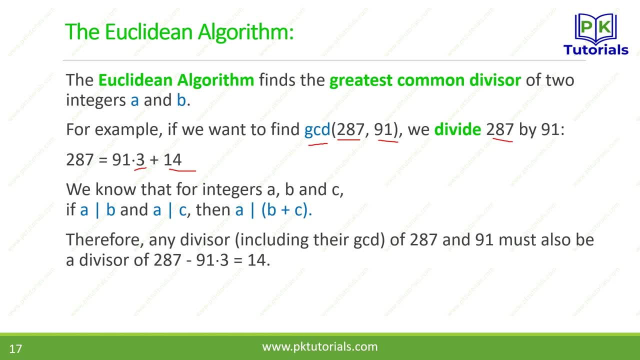 So if we subtract this, then this will also be its divisor. So, consequently, GCD of 287 is equal to 91, is equal to GCD of 14 and 91.. Now we will do the opposite in this. If we have 287 divided by 91, then the remainder of 91 is 14.. 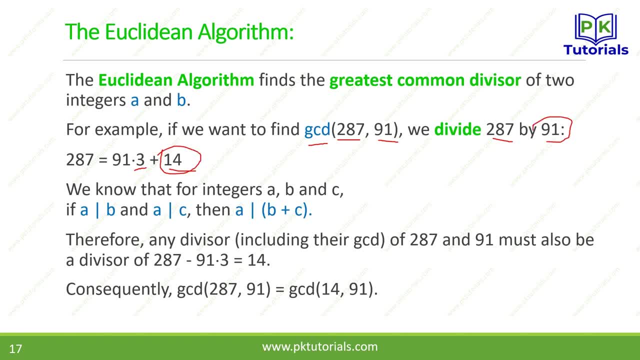 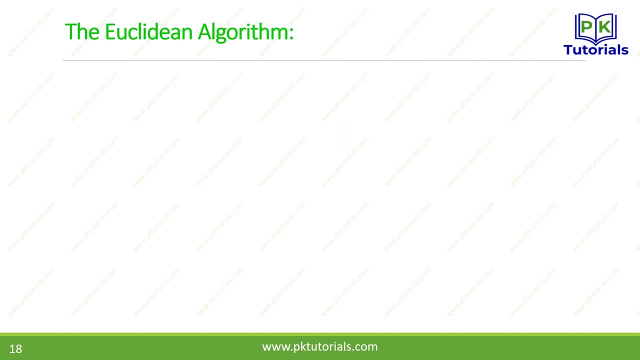 So if we take this with 91. Then GCD of 14 and 91 will be equal to GCD of 14 and 91. So on this formula, Euclidean algorithm's next step is to divide 91 by 14.. After this we have 7, and last time we had 14.. 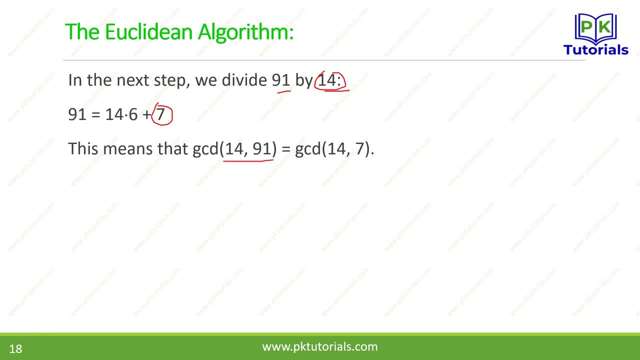 So now this means that GCD of 14 and 91 is equal to 14 and 7.. Now we divide 14 by 7. So we have 0.. Now, when we have 0. We find that 7 divides 14.. 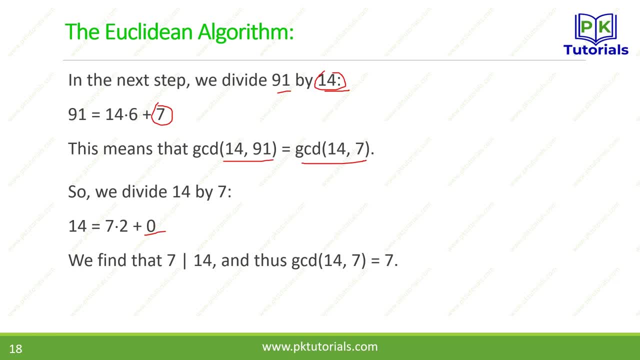 And thus GCD of 14 and 7 is equal to 7.. So we have the divisor of. its greatest common divisor is 7.. And this is Euclidean algorithm: that you do it stepwise. Whatever remainder you have divide the previous divisor on it.